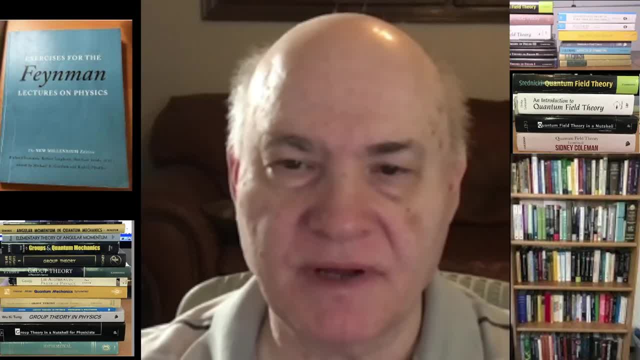 Hi, this is Mark Weissman. Welcome back to my YouTube channel. I wanted to make a video on just adding to my book list some pure mathematics books. That was a very popular video that I made on pure mathematics books for Physicist Entertainment. 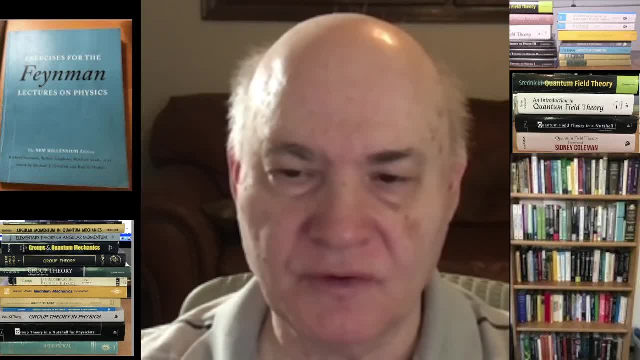 And in this video I'll add pure mathematics books on a topic that's probably my main interest in pure mathematics. I guess if I were to describe my main interest in pure mathematics, it would be foundations, which includes set theory, logic, recursion, computability, model theory. 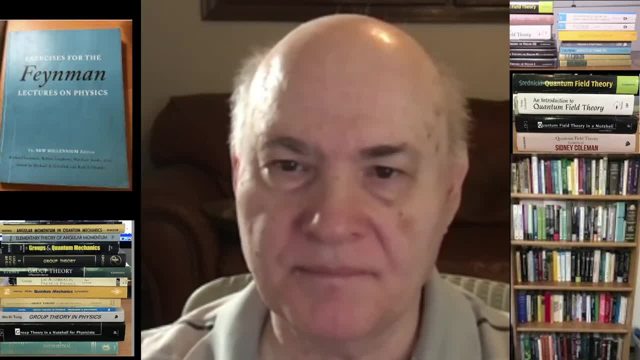 And then my other main interest would be number theory. Having said that, I'm going to add some books just that I own on the foundations in this video. Some of them will be repeat books that I had in the other video for Physicist Entertainment, but that's okay. 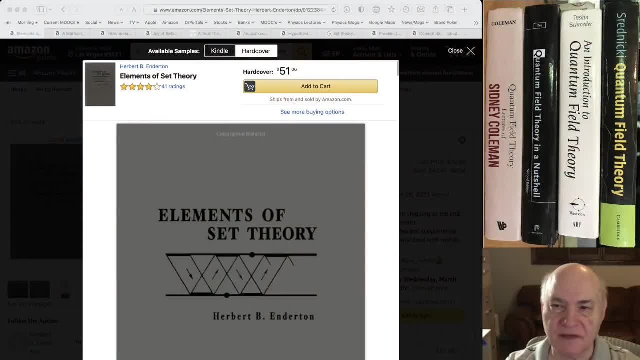 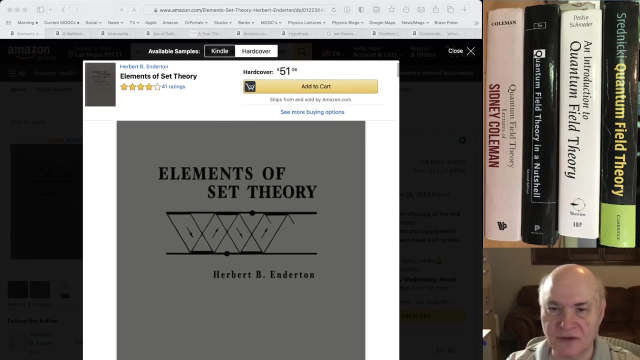 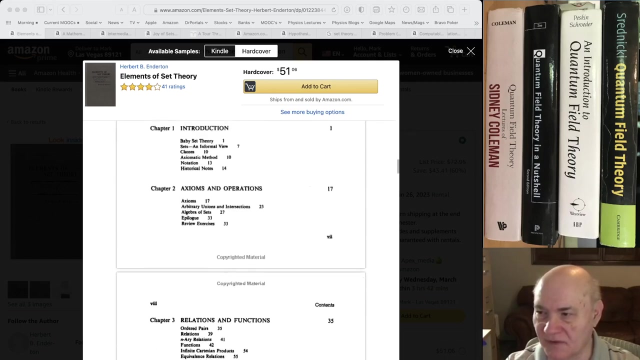 So if you're going to start out studying foundations, usually I would recommend you start out with some undergraduate books on set theory and logic. And this guy, Herbert Herbert Enderton, he wrote two excellent books. He actually wrote three of them, but the third one I don't think is that good. But he wrote two excellent books, undergraduate books. This is on set theory And you know it covers- I'll show you the table of contents in a second- but it's at an undergraduate level. It covers the you know ZFC system for axioms, you know, and it goes through developing the construction of the. 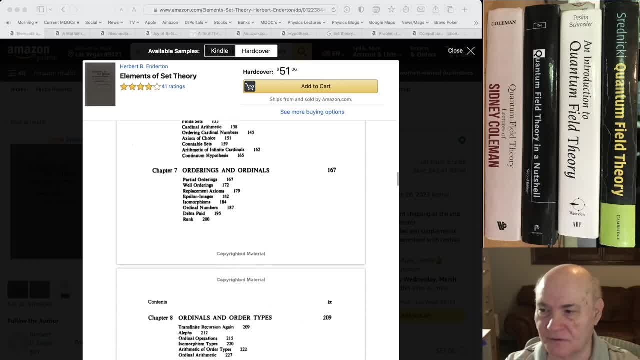 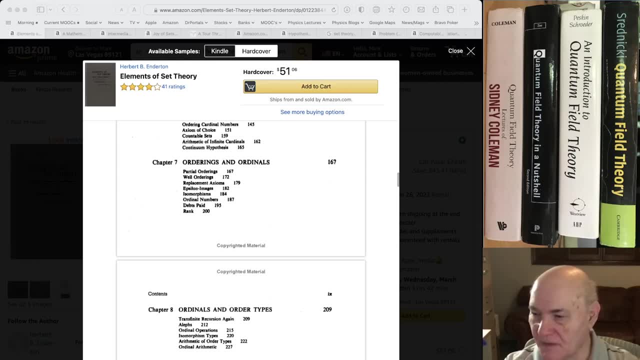 real numbers and everything and cardinals and ordinals and some special topics. As far as it goes, it proves the theorem on cardinality on. I can't remember the name of the theorem, but hold on, let me look it up. 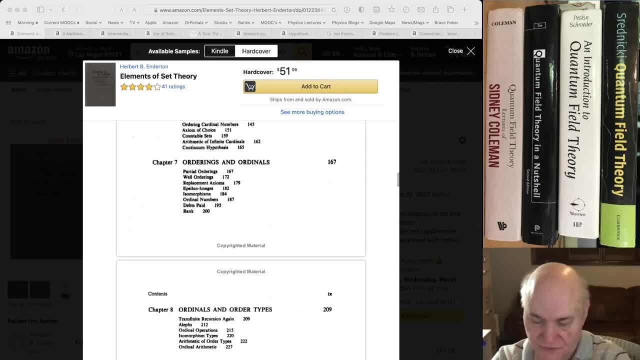 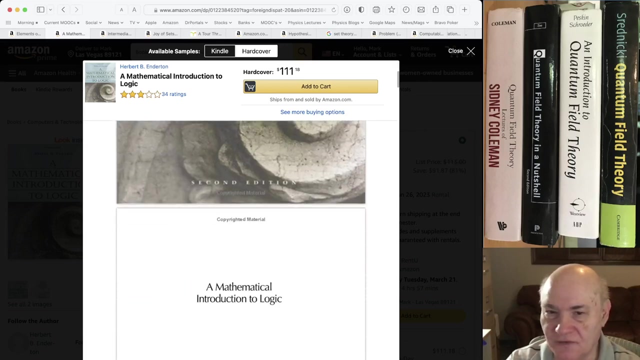 It talks about cofinality and Koenig's theorem, which is like the only theorem we have on cardinality. basically that says anything useful. So this would be my recommendations to start set theory and it's at the undergraduate level, a fairly easy read. And then he has a book on a mathematical introduction to logic. This is the best logic book that I found at the undergraduate level because it goes through all the details. 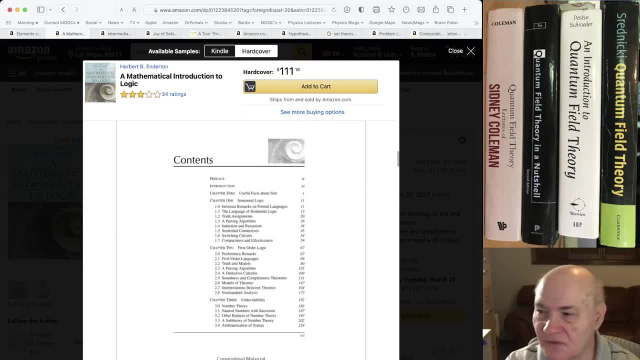 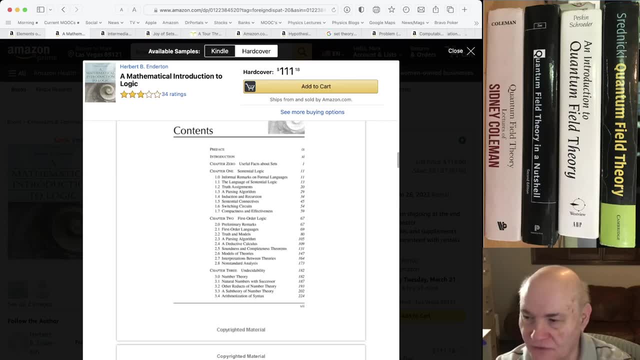 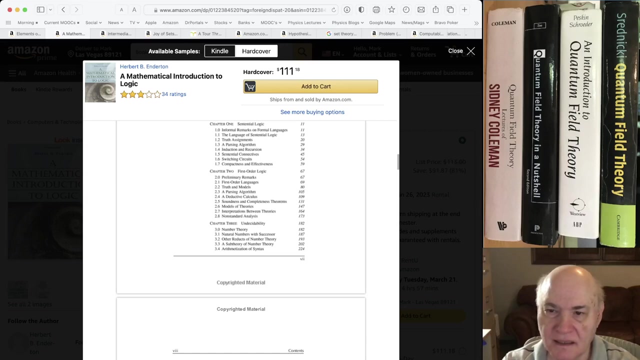 Most of the other books sort of say various things and skip a lot of details, but this one doesn't. It goes through all the details on, you know, recursion and representing functions and so on. It doesn't skip any details and it proves the incompleteness, theorems and undecidability. and it's I like this book as the best logic book because it covers all the details at the undergraduate level. 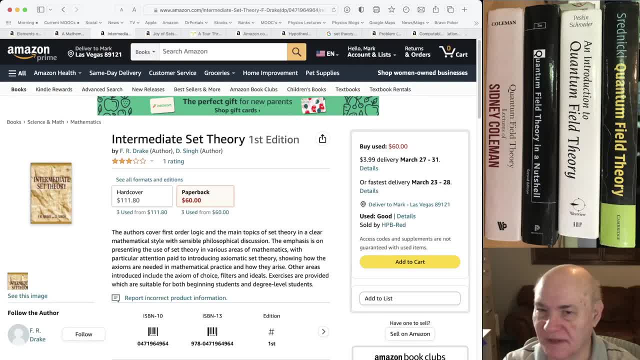 Now another book that I think I've mentioned before is a book called Intermediate Set Theory. This book- I can't look inside the book here, but this book also covers all the basic stuff in set theory, but it goes a little further to cover forcing and 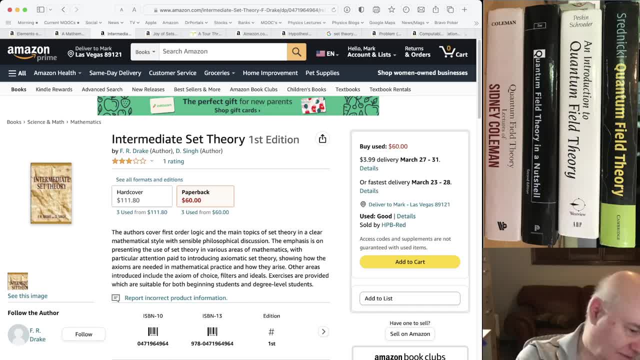 All of a sudden I can't find the books It covers- forcing And constructible sets and the independence things. So it's not an easy read. toward the end It goes through all these things on reflection principles and definability and absolute definability and everything. 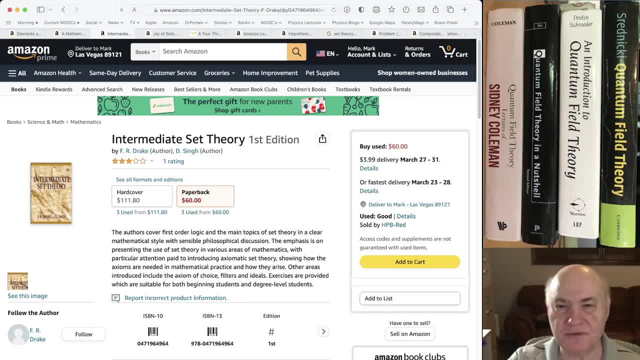 So I found this book. I got through the first. like two-thirds is fairly easy, but the last part, even though they give a lot of details, I didn't find it. It doesn't. It's not an easy read. 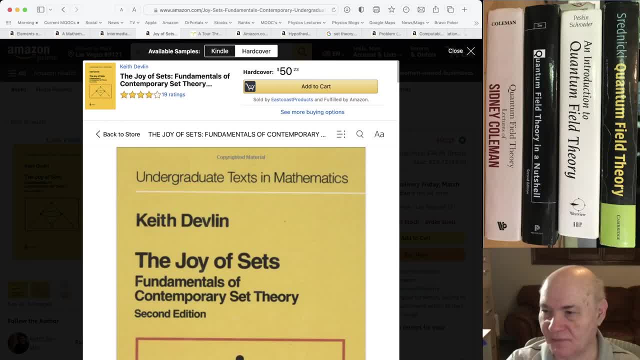 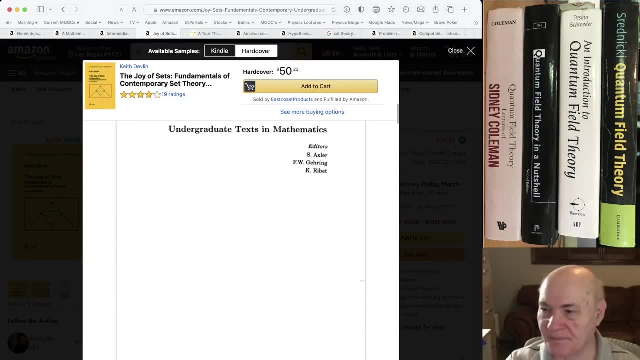 Another book that I have is The Joy of Sets by Keith Devlin. He's like a great mathematical writer of both popular books and textbooks, And this is one of the few books. He covers a lot of different things, but it's one of the few books. 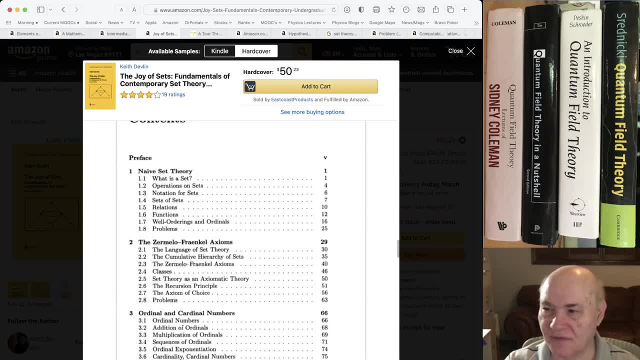 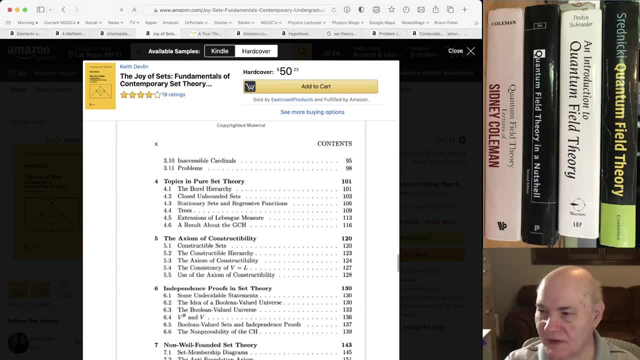 Let me get to the table of contents here. He starts off with naive set theory and then goes to the Zermelo-Fraenkel axioms. He covers a lot of the routine things, but then he does a lot of things. He doesn't give as much detail as other set theory books does, but he talks about things that they don't like. 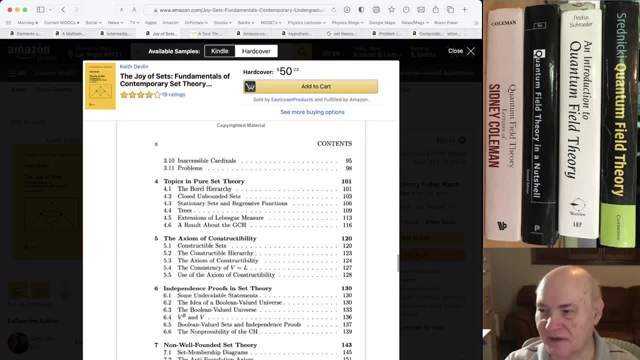 Even though he doesn't prove these things on constructability and independent proofs, he discusses them, And he's the only one I know who discusses the anti-foundation axiom. So if you're interested in that, which apparently has a lot of applications in computer science, you might want to look at that book. 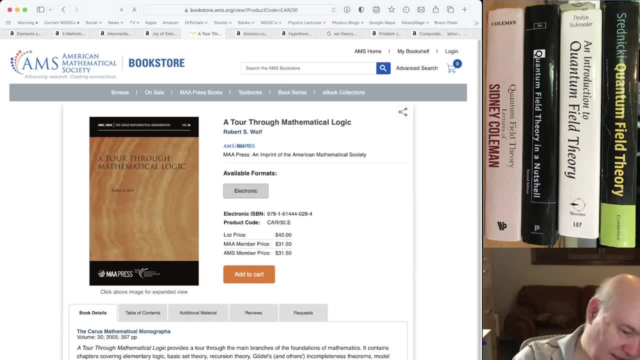 Now the next book that I have. This is: This is an interesting book. It's sort of seven-tenths Seven-tenths textbook and three-tenths popular books. It's like it says. The name says it's really a tour through mathematical logic. 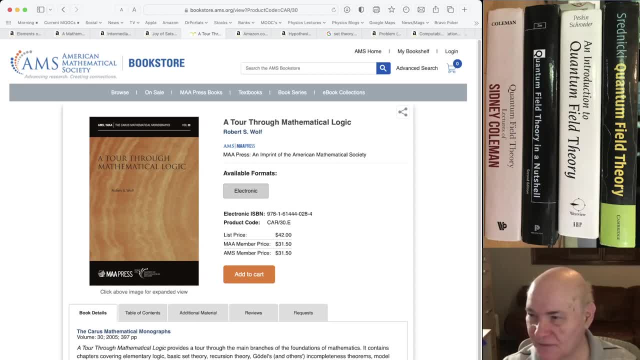 And for some reason on Amazon this is selling at an outrageous price. But on the American Mathematical Society who published it, their website is relatively cheap. I'll show you the table of contents. It's sort of routine. It doesn't really like prove anything. 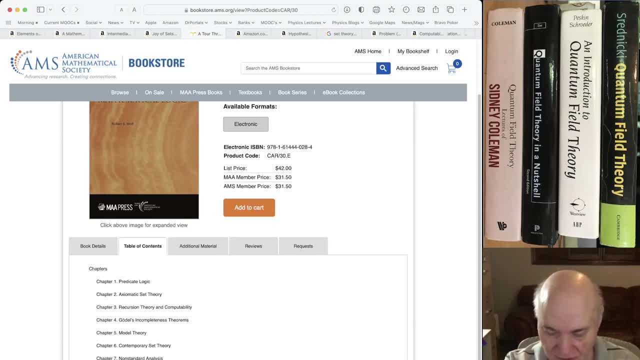 It sort of just states things, proves some things, But it really discusses a lot of the modern things like the Goodstein's theorem, the Paris-Harrington theorem, A lot of things in contemporary set theory, non-standard analysis and constructive mathematics. 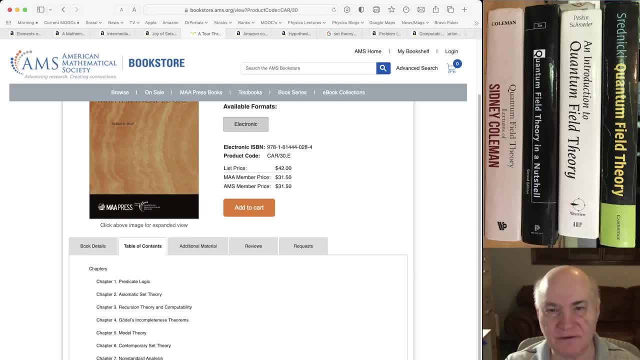 So if you want to have something to read about a lot of like results in set theory after you've studied it, this is an excellent book to read. It doesn't give the details, but it does give you a lot of results. 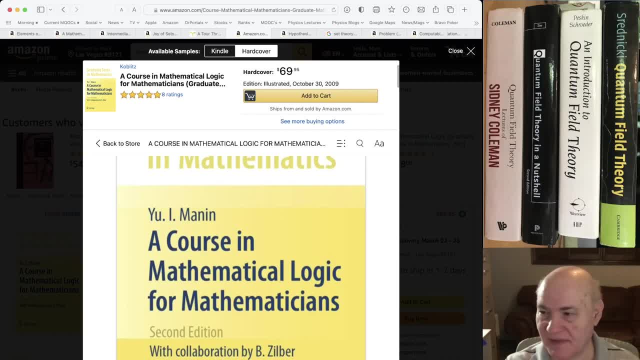 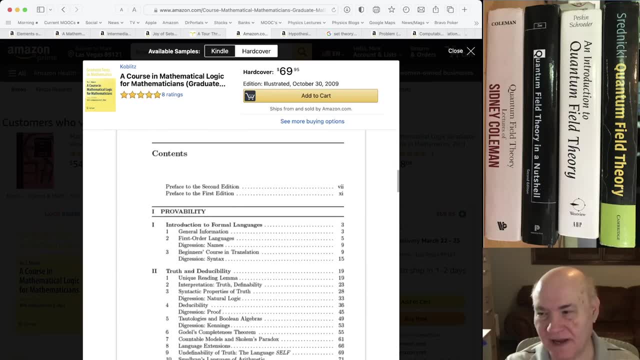 Now at the graduate level. this is a fantastic book by Mann and this is the second edition. He gives a lot of the details but it's at a graduate level and it goes quite fast. Once you've had like the undergraduate stuff, you can read this. 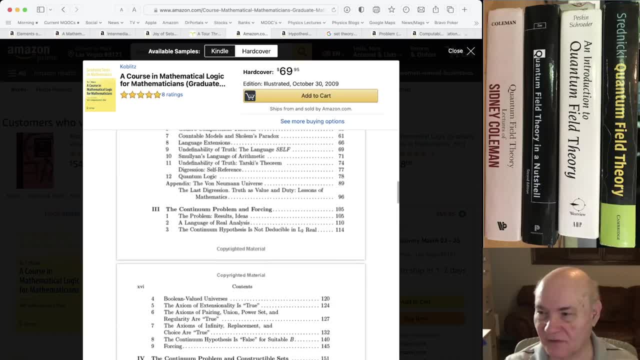 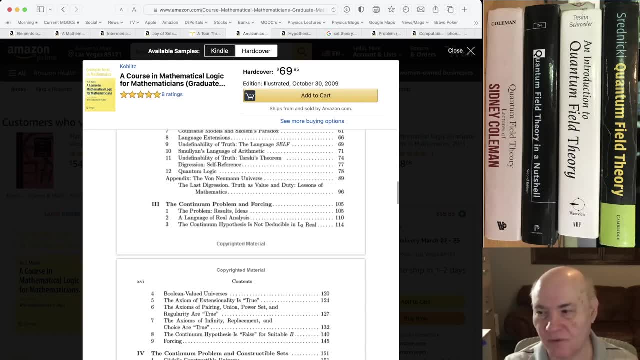 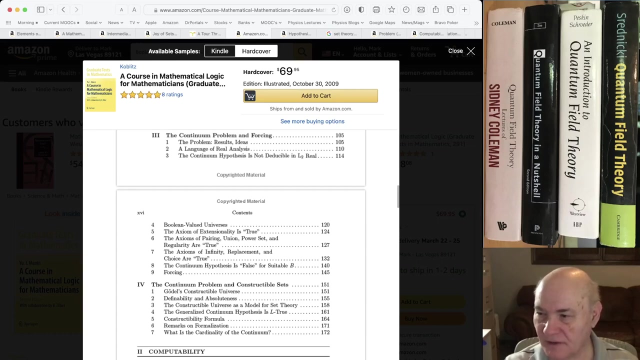 He starts with you know truth and decidability. It's mostly on logic. But then he has a chapter on the continuum problem and forcing and he shows you several different ways of doing it, one through Boolean-valued universe. So this is a really good book on giving you proofs on the continuum problem and constructible sets. 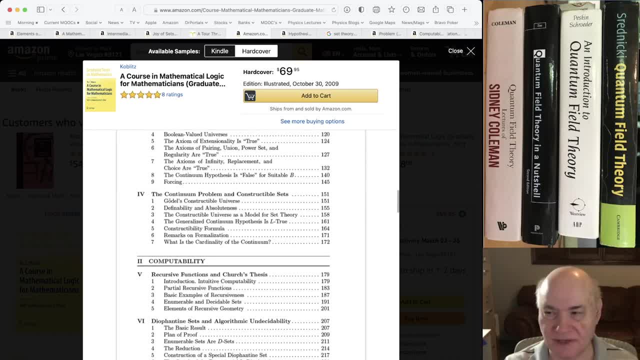 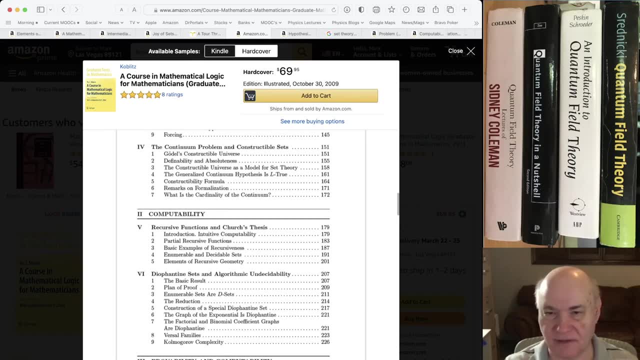 But then he has like two real fantastic chapters on basically Hilbert's 10th problem- recursive functions- and then he proves the Diophant and sets and algorithmic undecidability. It's the only place I've seen a really detailed discussion of this. 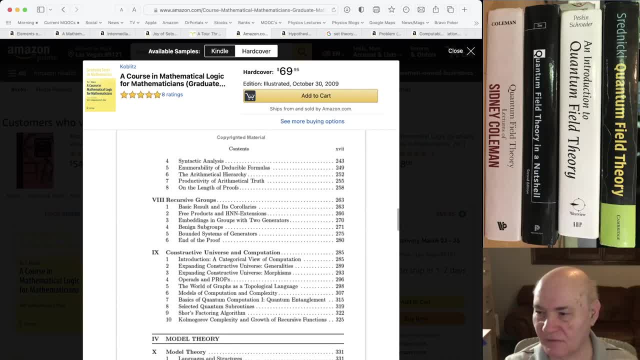 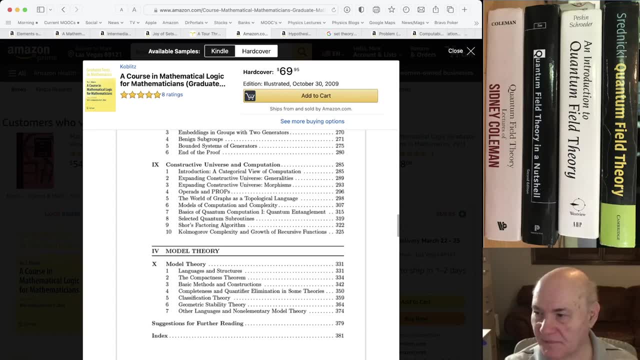 Then he goes back to Godel's incompleteness, results and recursive groups, and they added a chapter in the second edition. I have the first edition on model theory, So it's an excellent book. a lot of asides, He's a wonderful writer and the only problem is it's graduate level, so it's not that easy. 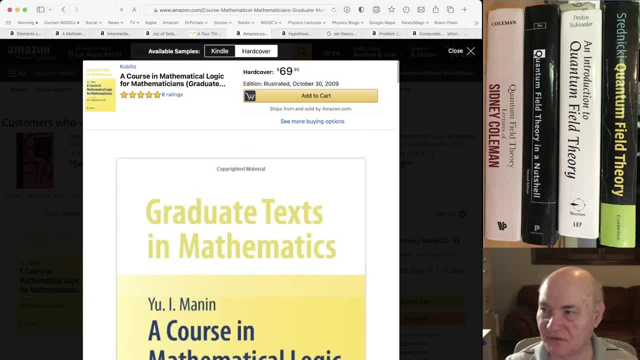 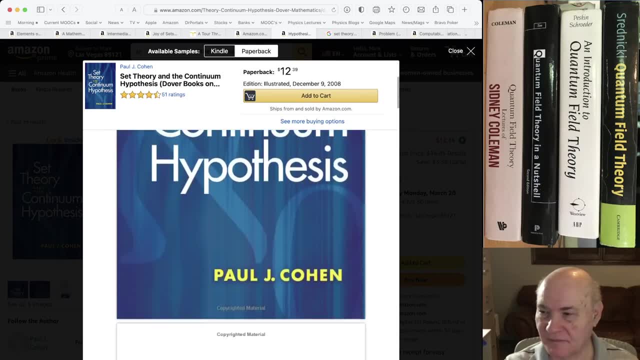 It's not that easy to work through it, but he covers a lot of different topics. This is a book I've only read about 20% of It's written by. I'm sorry, this is a book I've had a long time. 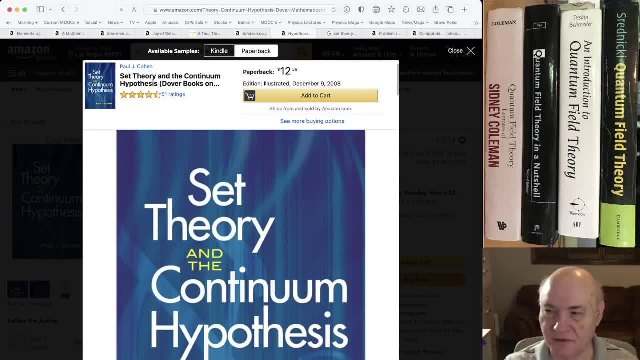 It's a Dover book, Set Theory and the Continuum Hypothesis by Paul Cohen. This was the original book he wrote in the mid-60s. The first third of it goes through, you know, set theory and predicate logic and everything. 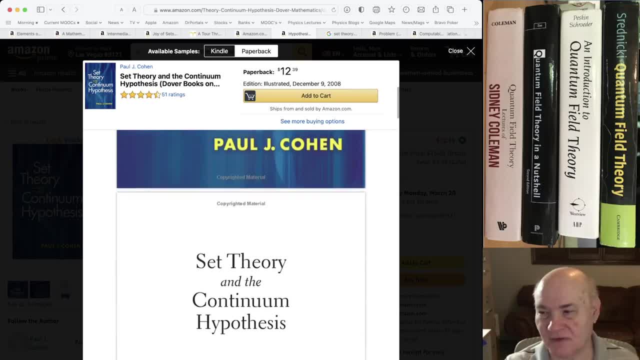 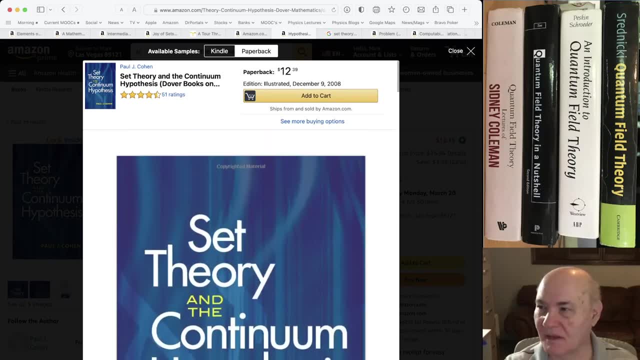 but then it goes pretty fast. Not that easy to understand. It's because I can't understand this that I bought a lot of other books to try and understand this. but one day I'm going to go through this again. This is like the original work in the mid-60s. 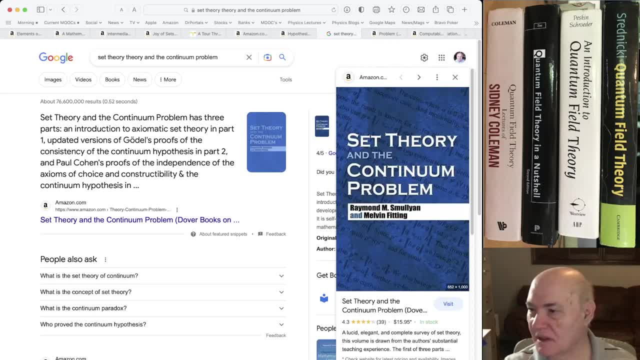 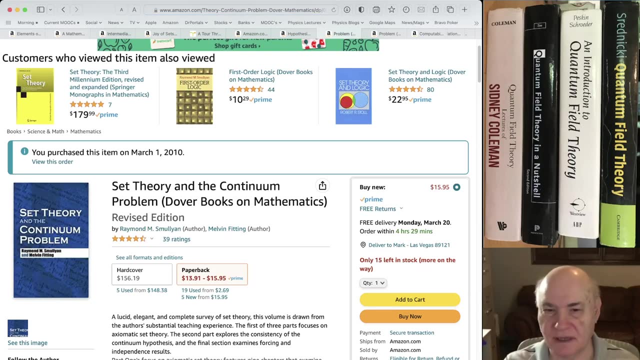 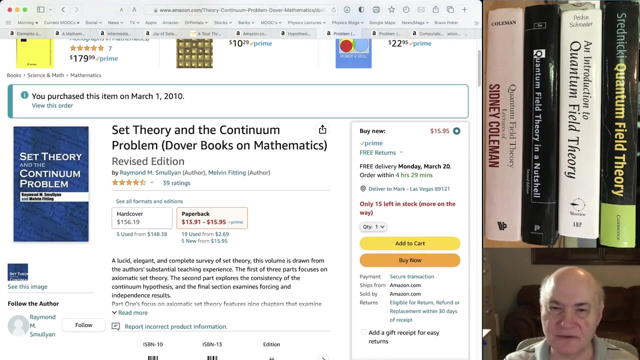 Now another book is Set Theory and the Continuum Problem. This is by Raymond Smullyan. Raymond Smullyan and another co-author. He's like the Feynman of logic. He passed away a couple of years ago, but he was like the expert on logic. 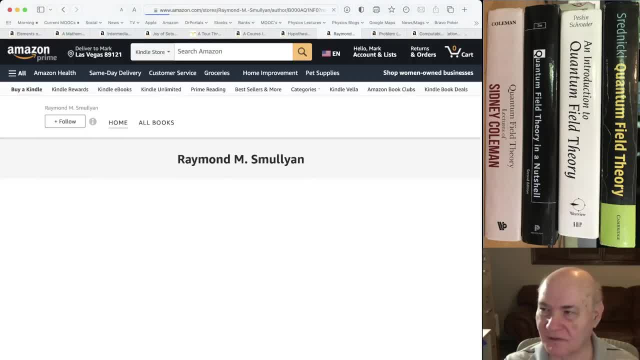 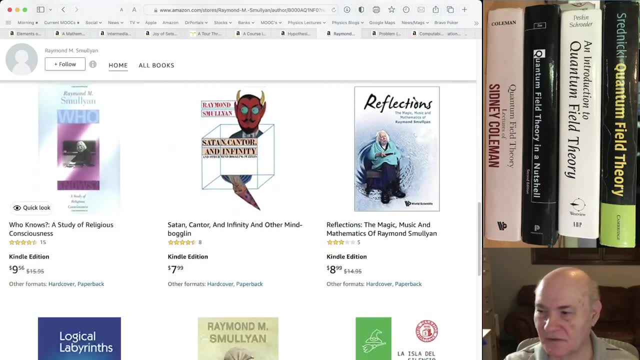 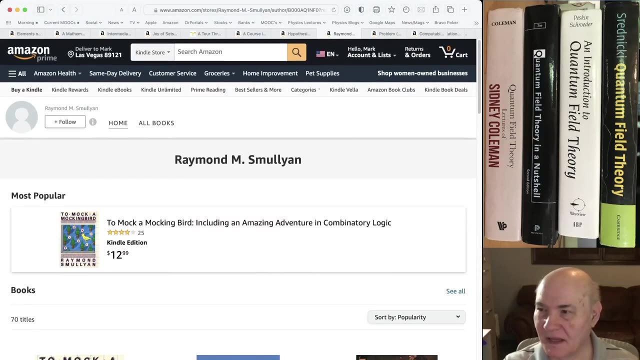 and he's written like so many books on logic. It's just like you know, many of them popular, some of them like about three or four standard textbooks and everything like Godel, incompleteness, theorems and everything. So, but this book, I thought I could get through it. 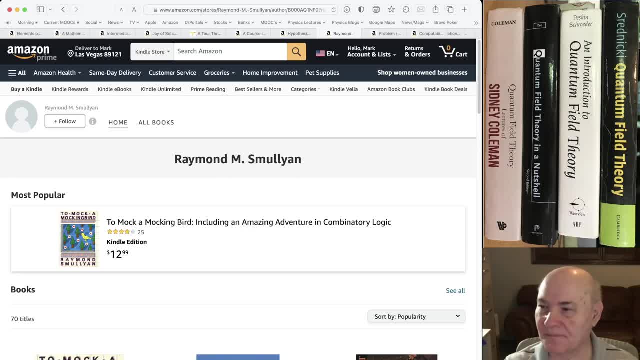 I got through about 20% of it and it's It's just difficult. But he talks about principles, like he has his own principles, like the super induction principle and everything and double induction and all these things. The word super in physics and mathematics always scares me. 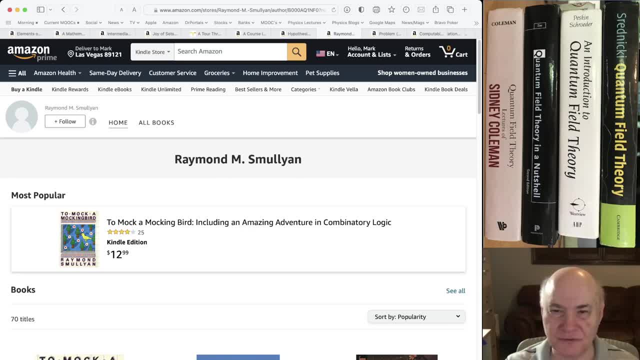 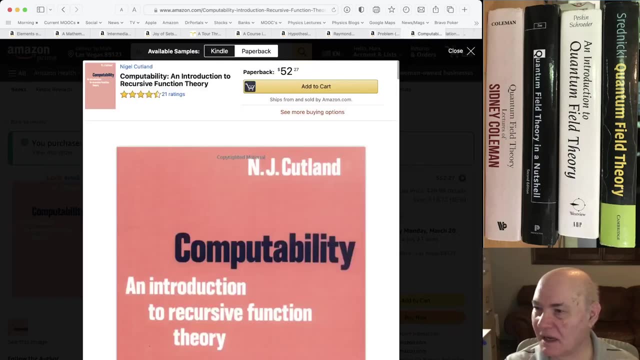 It can either mean super good, or it could mean super hard or super useless. So whether it's super string, super symmetry or super induction, you make your choice. So this was the book I just showed you. Now I only have one book on computability and recursive function theorem. 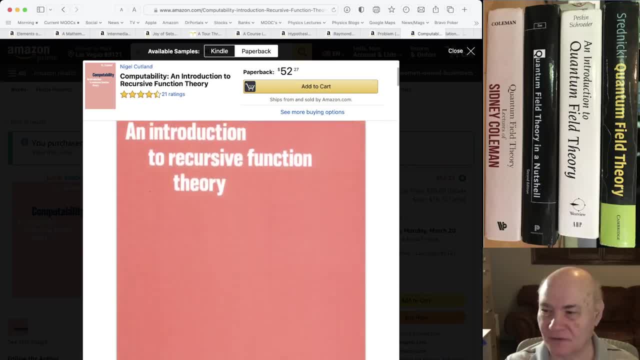 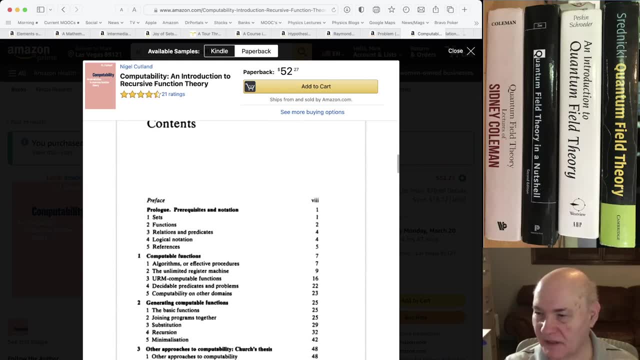 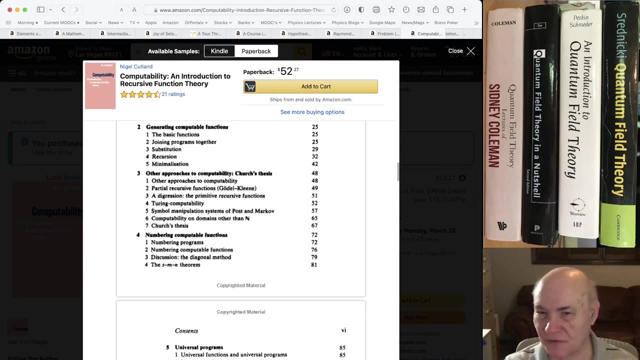 There are others, There are better ones. This is an easy book to read. It's by Cutland and he sort of uses the register model and it's an old book, or at least goes back to the 80s, But it's easy to prove and he goes through things like primitive recursive. 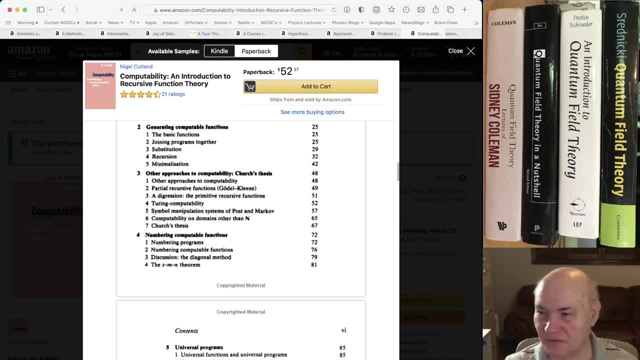 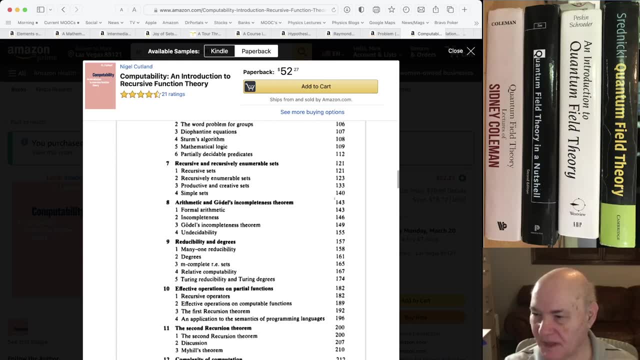 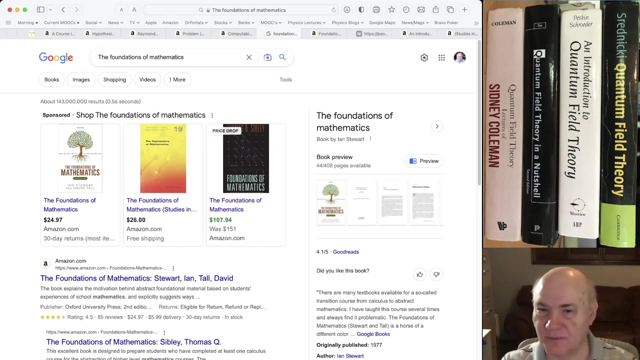 and Ackermann's function, which isn't primitive recursive but is recursive. He covers a lot of interesting things on effective computation and everything, So it's well worth reading and it's easy. Now the next book. I found these books recently, I'm sorry. 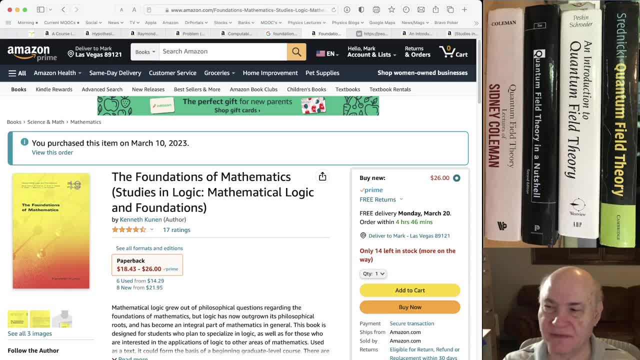 on The Foundation of Mathematics by Kuhnian. Since I want to restudy this and I don't want to read all my old books again, this is a very cheap like $18 to $26.. It's by a renowned author, Kenneth Kuhnian, and I'll show you a standard book that he wrote. 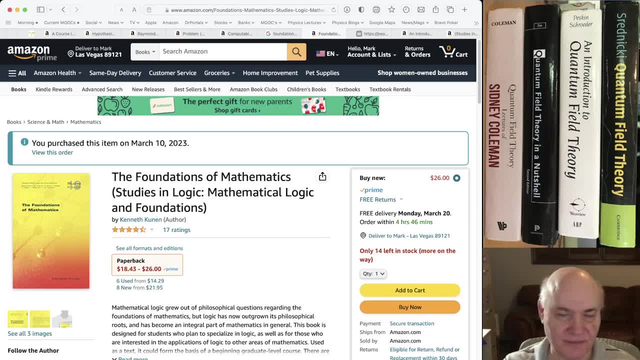 And in this book he covers the foundations of mathematics. He basically has three chapters. It's about 270 pages. He has like basically three chapters: One is on set theory, one is on logic and one is on recursion. And it's sort of like at a graduate level and the idea is to get you to be able to read his other books. 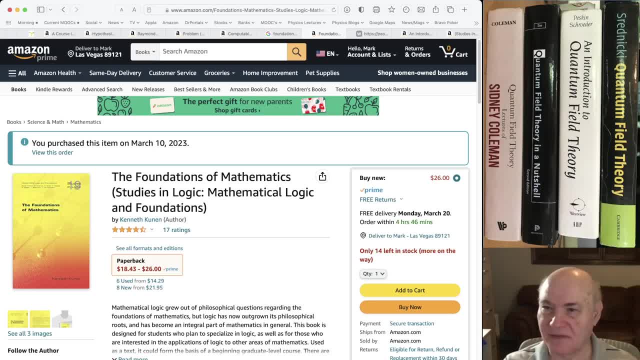 So I really recommend this. if you've had set theory and you've had mathematical logic, I would recommend that you read- and you don't want to read the same books over again. You might want to consider reading this book. See, I've already started reading it and I'm about 50 pages through, and it's really excellent. 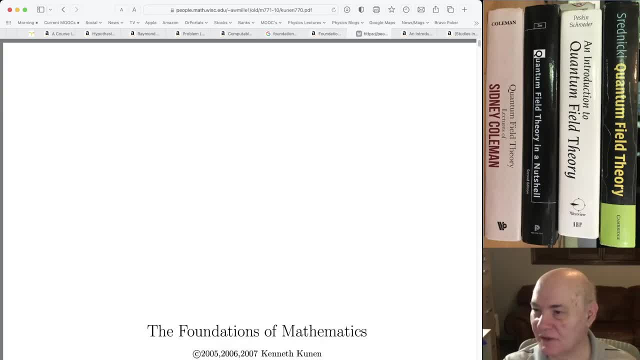 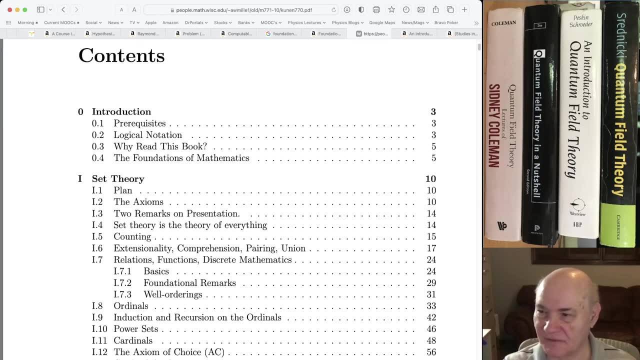 He's an excellent writer. Now he's also the author of. by the way, you can get a draft of this book. It's not complete. It only has like the first two chapters online. If you just Google, you can get a graph of it. 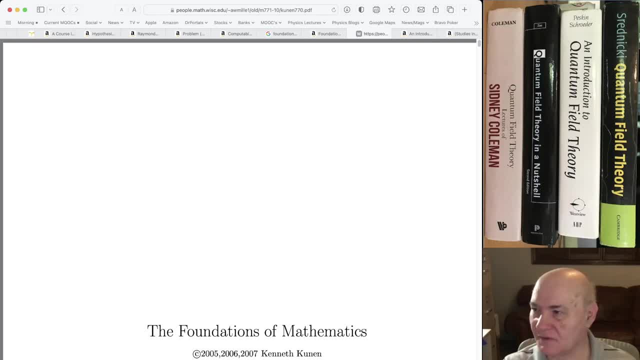 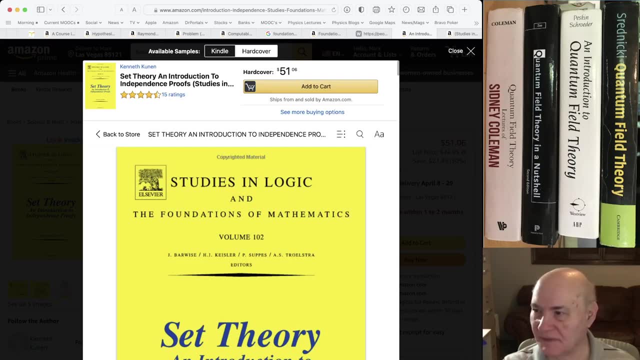 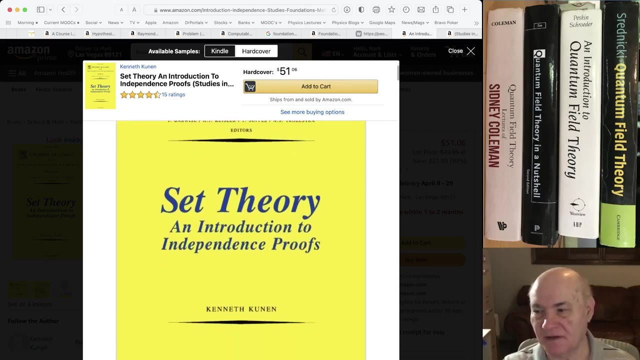 But it's not the same. but just in case, This was his standard book from a long time ago and it's kind of like you know it's $50.. It's not that cheap, not that expensive. Set theory, an introduction to independence proofs, but it's old. 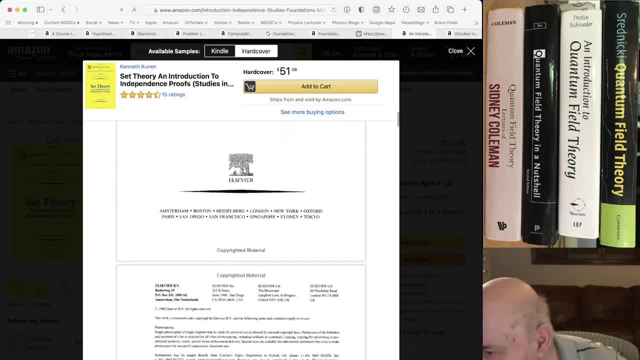 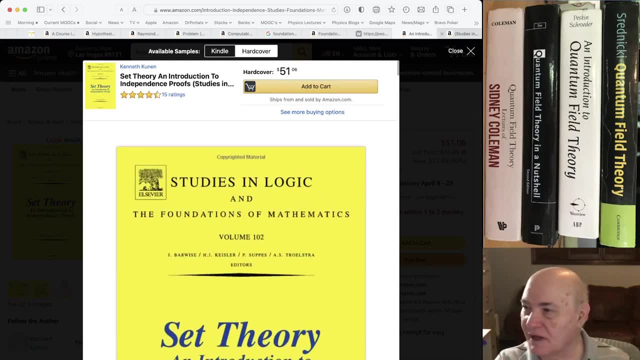 It was published in like 84, or let me see when it was published: 1980.. So he's updated this book and he's got a new book and it's called Set Theory: Studies in Logic. It's a cheap edition. 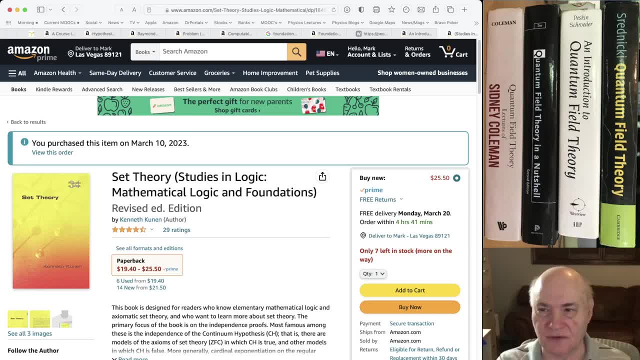 And in this book he proves all the independence results and he uses forcing. He doesn't use Boolean algebras or anything. But I highly recommend this book. It looks like it's accessible. If you want to read about this kind of stuff, Kunin is like your go-to guy. 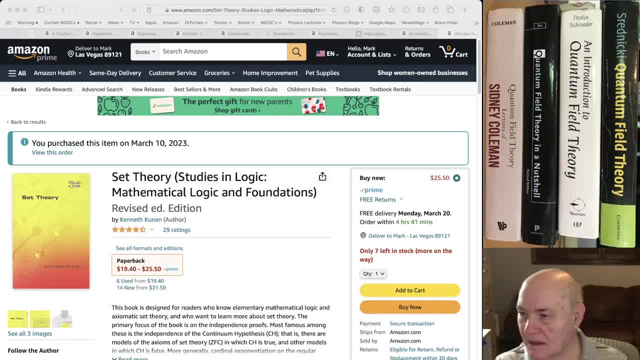 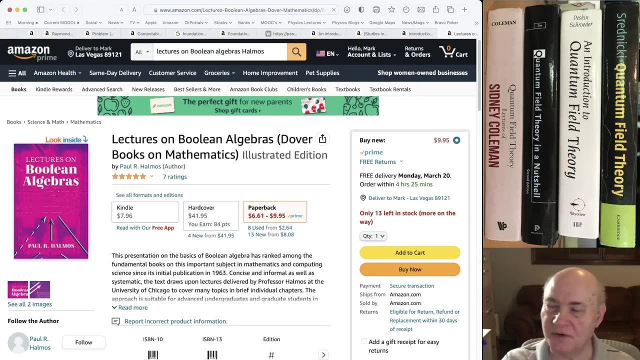 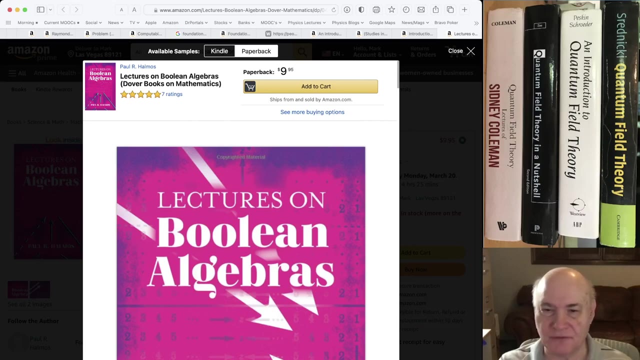 And I highly recommend it. Now there's a couple of other books. So some of these books like Manon's book. they take a Boolean algebra approach. There's two main approaches to this whole set theory and independence proofs. One is Cohen's forcing method and another one sort of bypasses that and uses Boolean algebras. 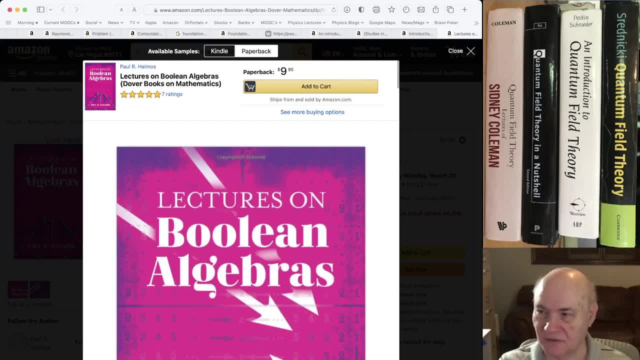 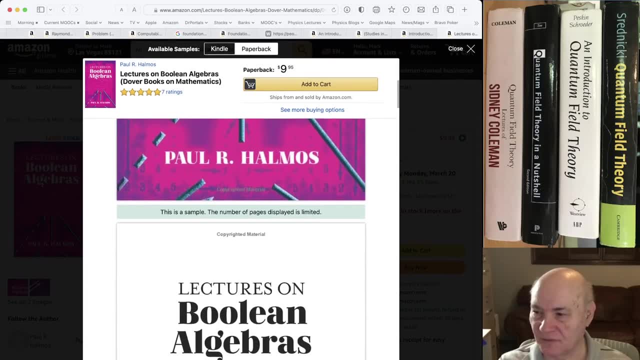 It's hard to find a good book on Boolean algebras. There's an old book by Paul Halmos, very cheap, It's like $9, $10. It's lectures on Boolean algebras. It goes back to the early 60s. 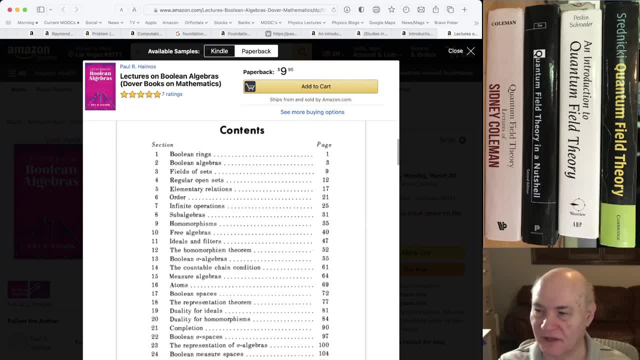 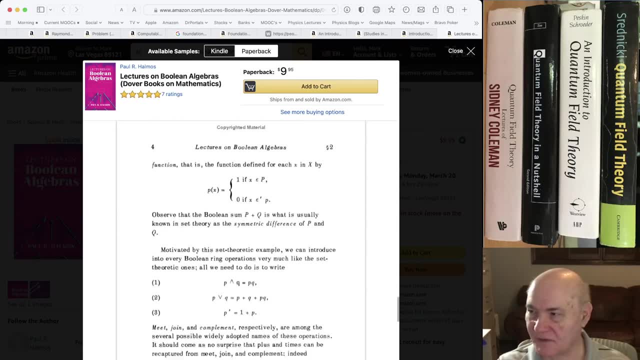 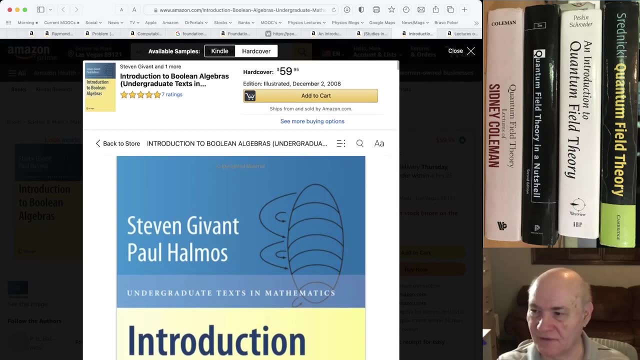 And he covers everything you need on Boolean algebras to understand probably these set theory books. But this one's like fairly terse. You sort of have to figure it out yourself. Now he has another book. They updated this book. This is an undergraduate book in mathematics. 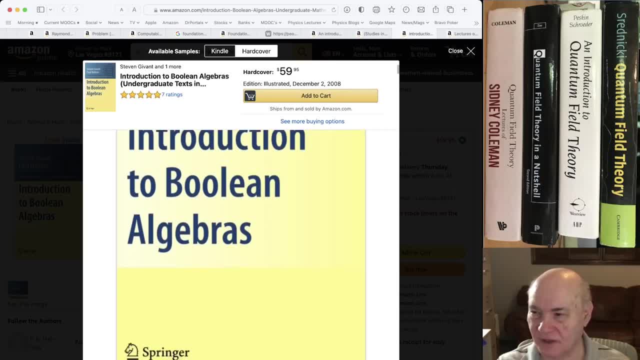 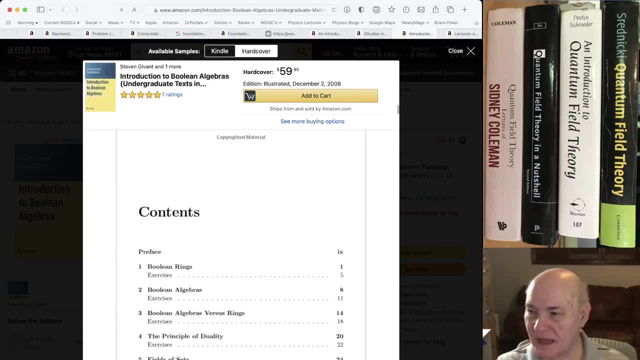 It's the same book basically, except with all the details. This is three times longer. Introduction to Boolean Algebras: It's like $60, standard spring a hardcover And you can see. the chapters and everything are the same, but it's like three times longer. 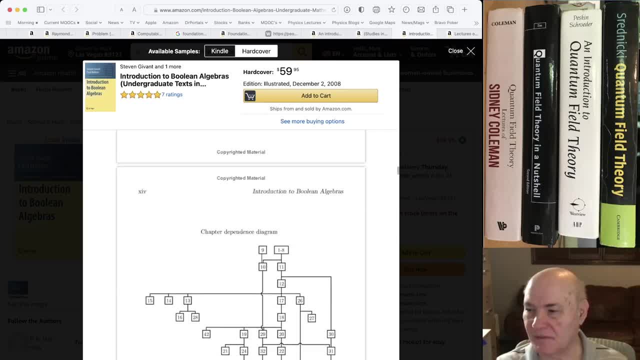 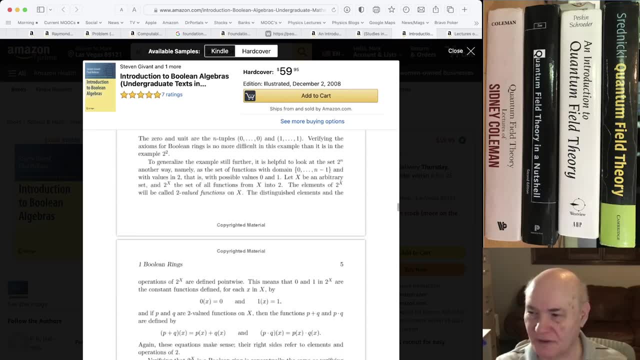 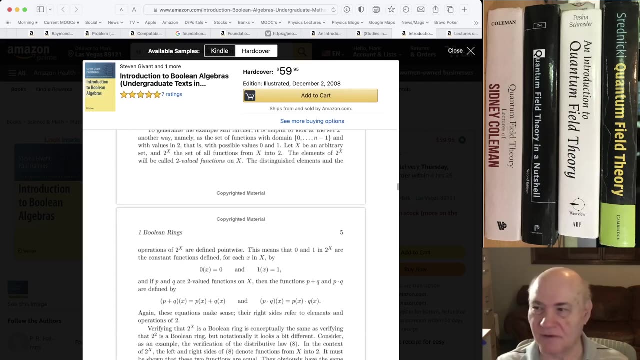 You know, if you read the preface you'll see what I mean. But you know, he just proves everything. What things that he leaves out of the other book. he proves in pretty good detail and it's pretty easy. So if you want to get a book on Boolean Algebras, I highly recommend that.